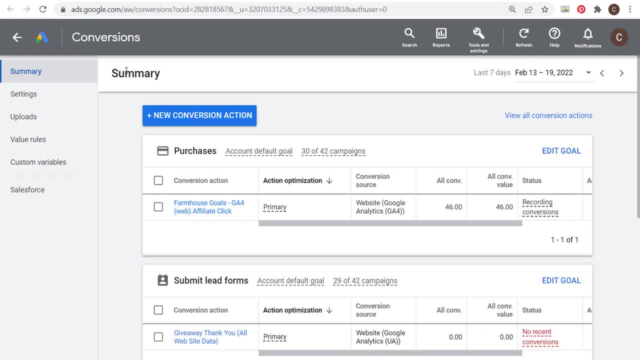 conversions, and that's going to bring you to the conversion actions page, And what you can do here is create new conversion actions or make sure you're optimizing for your existing conversions. The best way to get the most out of Google Ads is to use conversion tracking and to continue to. 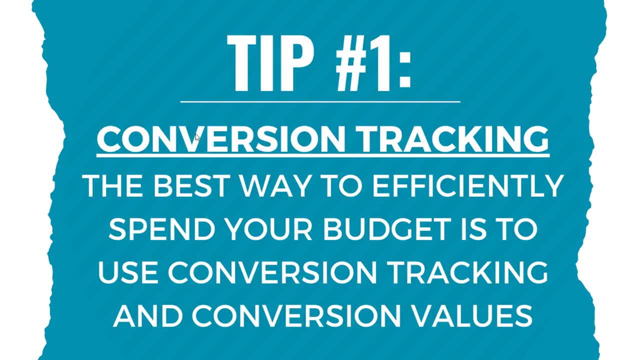 optimize your campaigns over time. So, if we come back over here, if you want to spend your budget efficiently, you can do that by clicking on the conversion actions page. So if you want to spend your budget efficiently, you need to understand how your campaign is performing. I'm going to 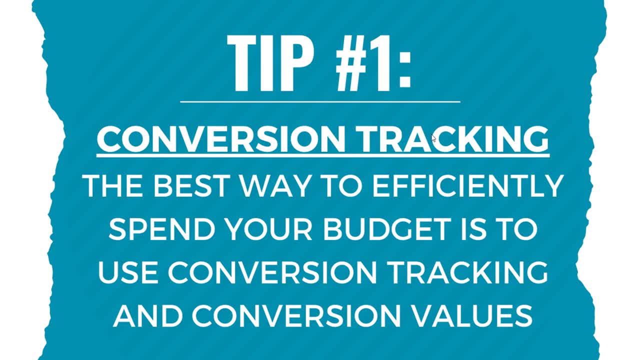 create a separate video about conversion tracking and conversion values and really everything you need to know about that. But for right now, what you really want to do is, if you want to spend your budget efficiently, you want to use conversion tracking. So that's tip number one. Now tip: 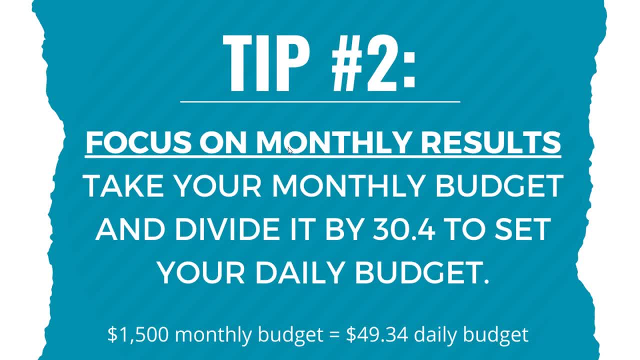 number two is to focus on your monthly results, And what you really want to do is set a monthly budget ahead of time and then use that monthly budget, divide it by 30.4 to set your daily budget. So you could see right here: if I had a $1,500 budget, I would be able to set a monthly 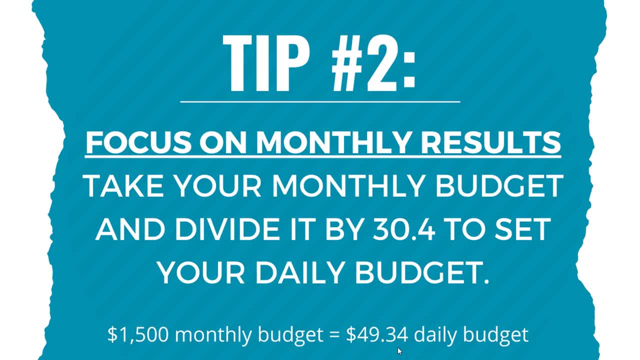 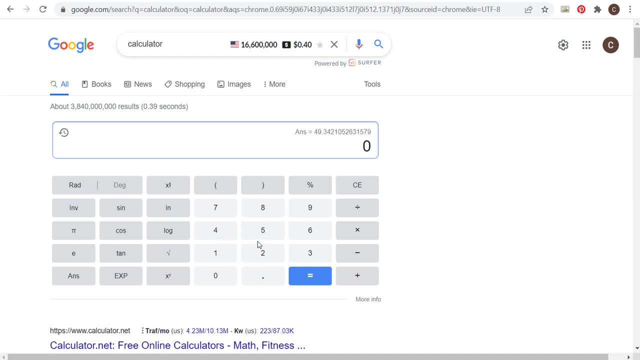 budget. That means my daily budget should be $49.34.. So if we come over to our calculator here- and you can see I was just doing it in here- but if you have any budget you set, so if you have $2,000 budget- all you want to do is take that budget, divide it by 30.4 and click on equals. 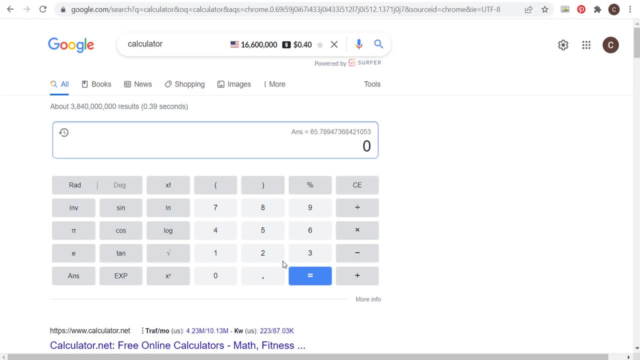 And that's what you want your daily budget to be around. Now, if you say: I know I want to spend $25 per day, then take that number, multiply it by 30.4, click on equals and that's how much. 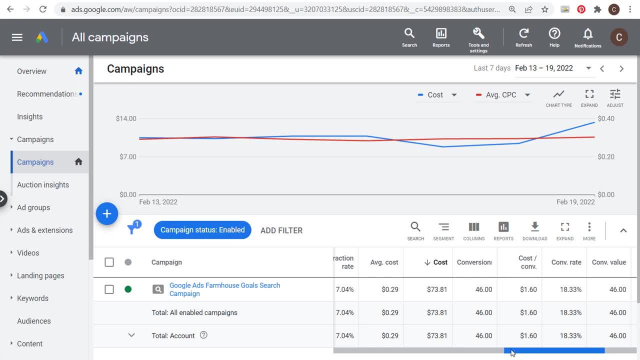 you're going to spend for the month. So if we come over to my campaign and I scroll over, I have a $10 daily budget set. So you can see, in February I won't be charged more than $304 for this campaign. So the way Google. 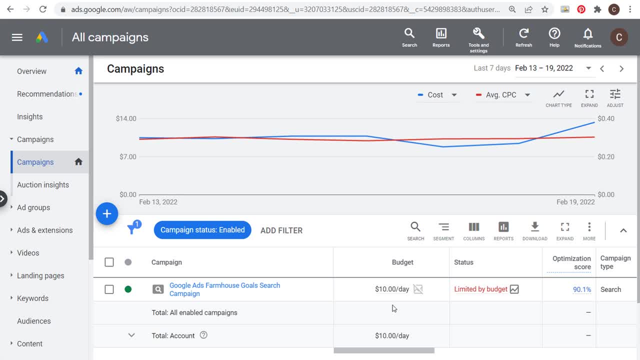 ads works is when you set your budget. Google is really looking at driving you the most conversions over the course of a month, So they're going to try to get the most out of each individual day. But if you're changing your budget and going up way too much too, 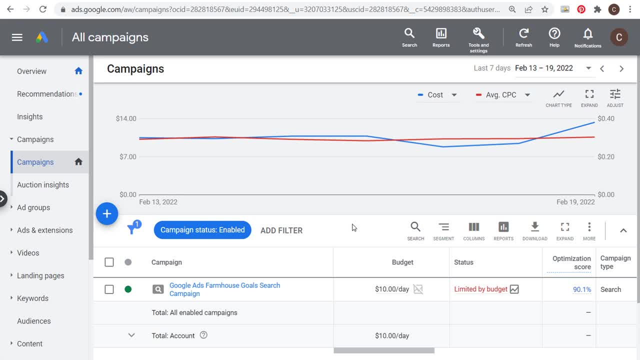 often, or going up and down and kind of bouncing all over the place. it's going to hurt your overall results with Google ads, because what Google ads is doing is saying, okay, today we're going to spend $8 and 79 cents because we think we can actually drive more conversions based on 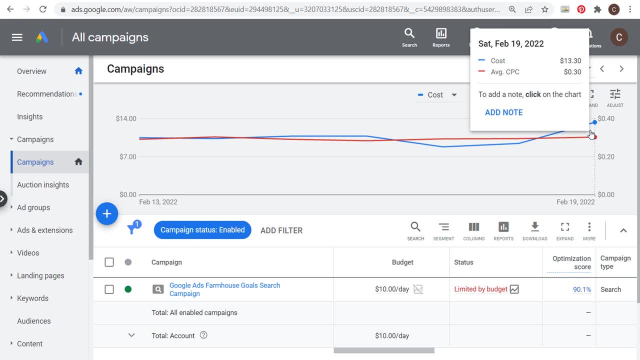 historical data on Saturday, where we're going to spend $13 and 30 cents- And you'll see bigger swings the higher your budget is. So if you have a $500 daily budget, you might spend $600 one day and you might spend $400 the next. So what you want to do is make sure you're focusing more on 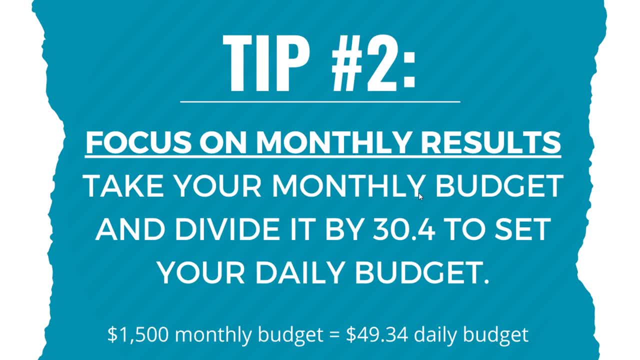 your monthly results and you don't want to be changing your budget too often. So if you're focusing more on your monthly results and you don't want to be changing your budget too often, I would highly recommend keeping your budget pretty similar And if you are going to increase it or 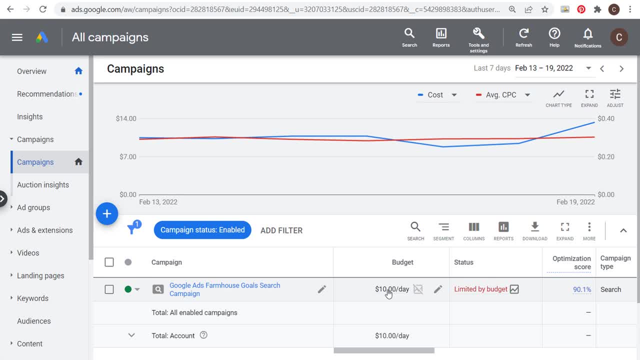 decrease it. do it gradually. So go from $10 to $15, from 15 to 20.. Don't go from $10 to 50, back down to 10, because all you're doing is messing with Google ads and how much they're planning on. 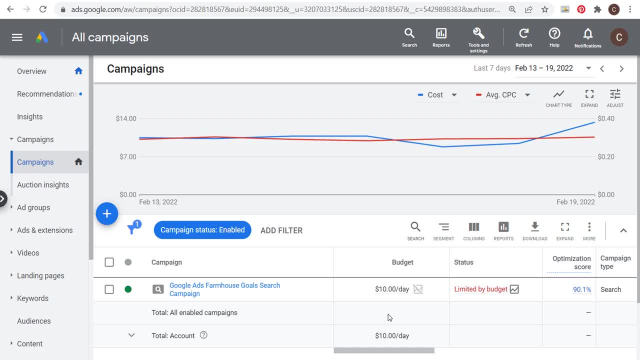 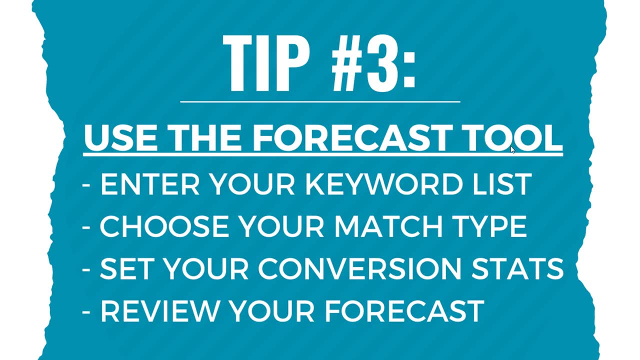 spending for your campaign over the course of a month And it's going to hurt your conversion results. Okay, So next is going to be tip number three. So for tip number three, you can use the forecast tool in the Google keyword planner. All you need to do is make sure you have a keyword. 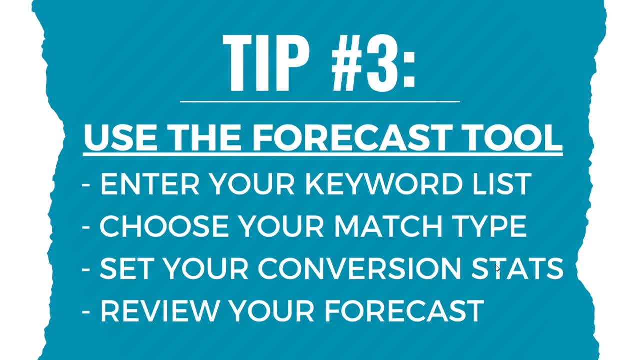 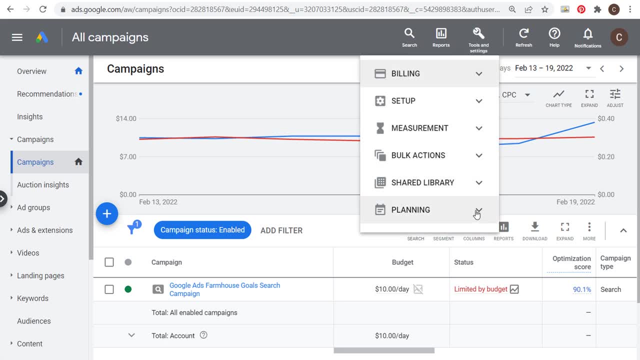 list. You need to choose your match type, set the conversion stats for your overall website and then review your forecast. So if we come over here and we click on tools and settings, we go to planning and we open the keyword planner. You can see, I have it open here. 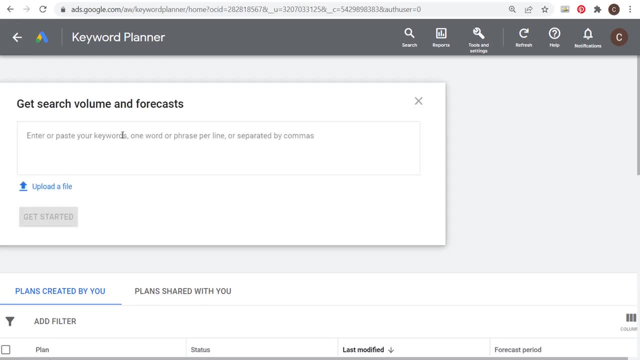 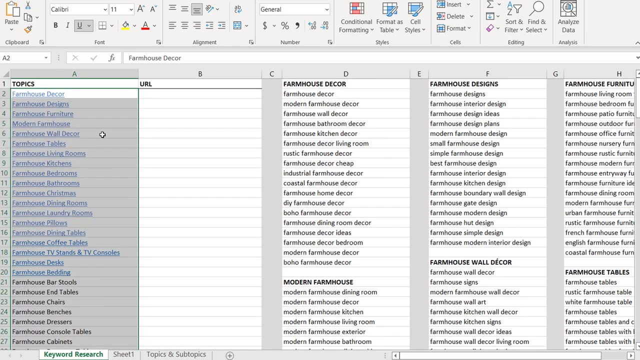 What we want to do is click on get search volume and forecasts and we want to paste our keyword list here. So if I come over, I have my keyword list open here in this Microsoft Excel file. I've copied the entire thing, So we're going to copy it. come back over and we're going to paste this. 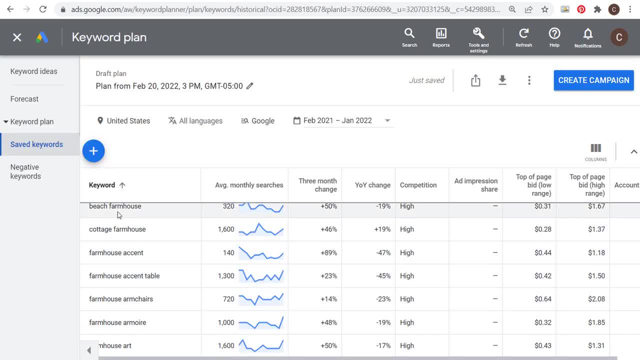 Click on get started. So, first, what it's going to show you is the keywords that we entered: average monthly searches, three month change and you get all this data over here. But what you want to do over on the left-hand side is click on forecast. So what this is going to do is it's 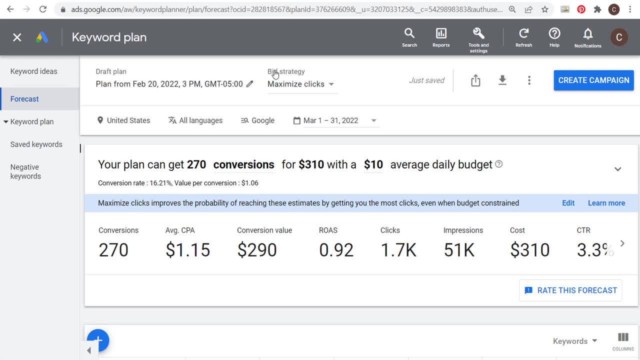 going to create a draft plan campaign. The bid strategy is going to be maximized clicks and we're looking at forecast data for next month. So I'm filming this video right now. It's February 2022.. So it's giving me forecast data for March 2022. And you can see here it's showing 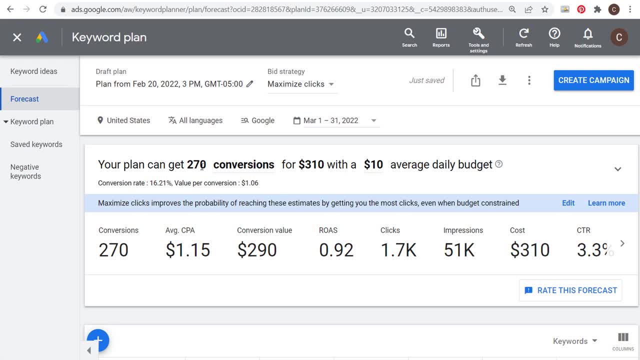 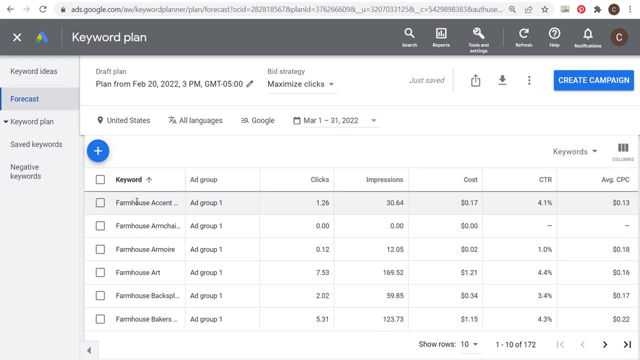 if I have a $10 average daily budget, I can get 270 conversions for $310.. My total conversion value would be $290.. My total cost would be $310.. So let's change the data around a little bit and let's set our match types. So the first thing we want to do is we have all of our keywords here. 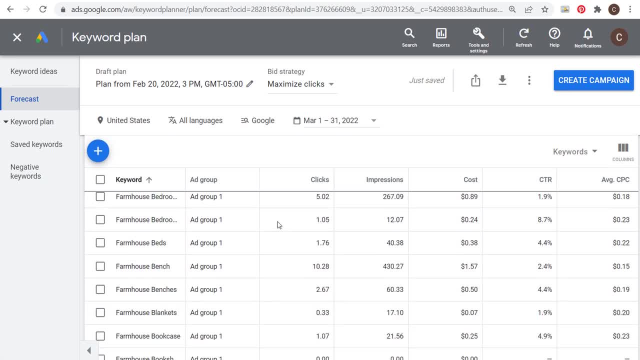 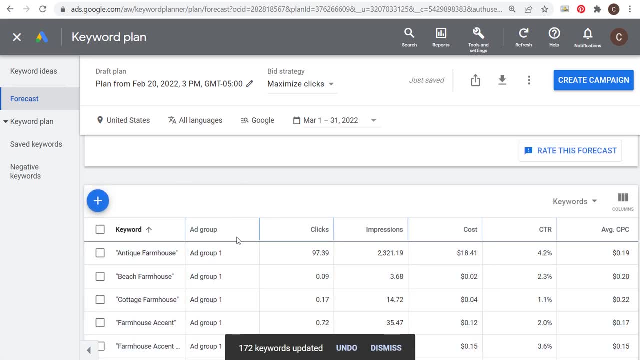 We want to click on show rows 500, so we can select all of our keywords at once. We're going to select all of them, edit our match type and choose phrase match Targeting, phrase match keywords. So you can see our conversion value actually went down slightly. 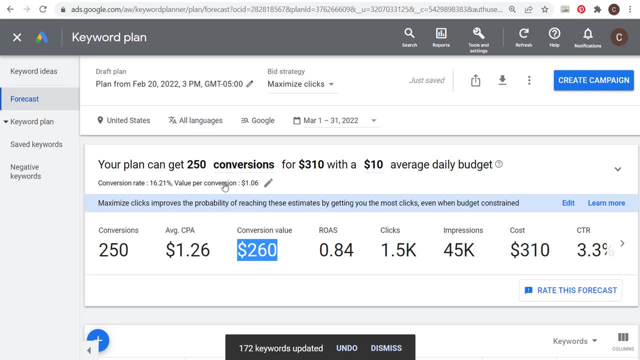 but what we want to do next is, if we click right here, you can see conversion rate and value per conversion. So let's just say, for example, my conversion rate historically is 7% And let's just say my value per conversion is $5. So we'll do 7% and $5 and click on save. So right now, 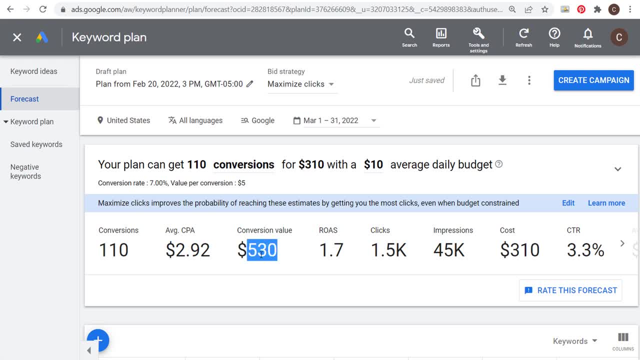 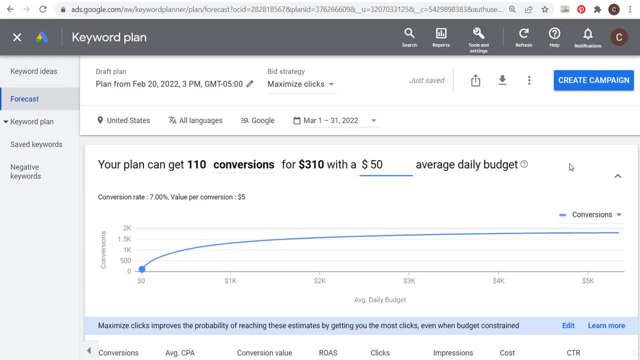 what it's showing is my conversion value would be $530 and my cost would be $310.. What we can do is say, okay, let's say I want to spend $50 per day, So we'll set it at $50 per day. 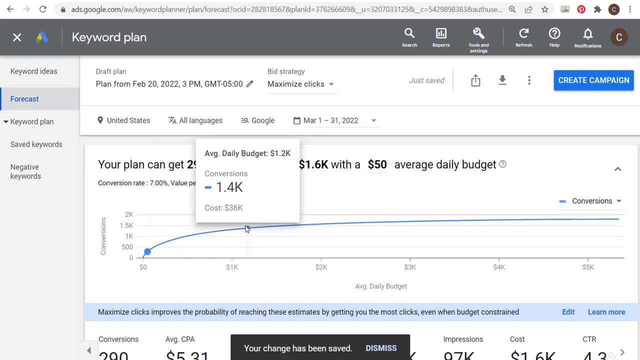 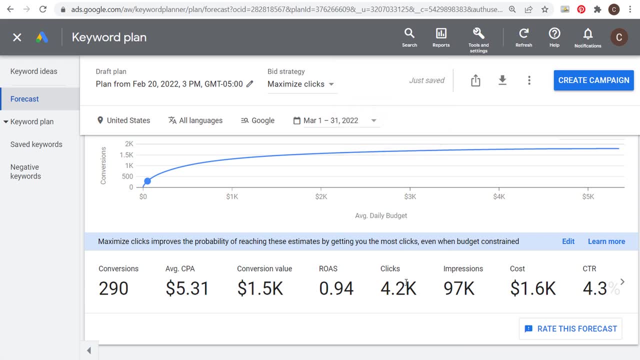 and you can see this chart right here. You can actually adjust it. So it's going to adjust your average daily budget and show you how many conversions you can get. But if I'm choosing a $50 average daily budget, it's saying I'm going to spend $1,600.. My conversion value will be 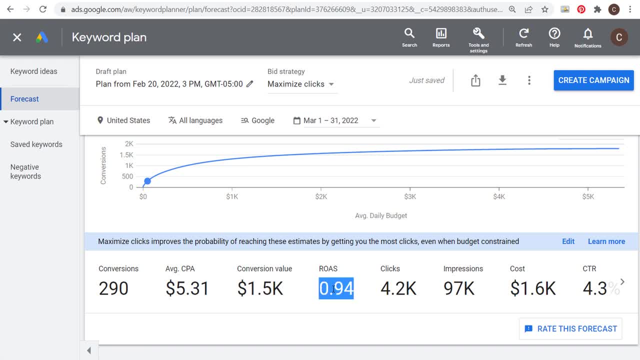 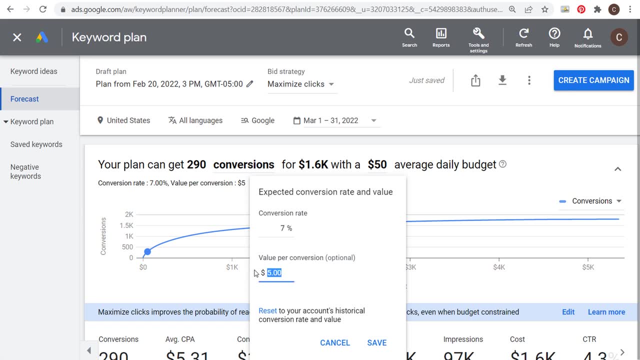 around $1,500.. My return on ad spend will actually be less than my break-even point, so I'm technically not making money on this campaign. But let's just say my value per conversion is $7.. Let's say my conversion rate is $8.. We click on save. 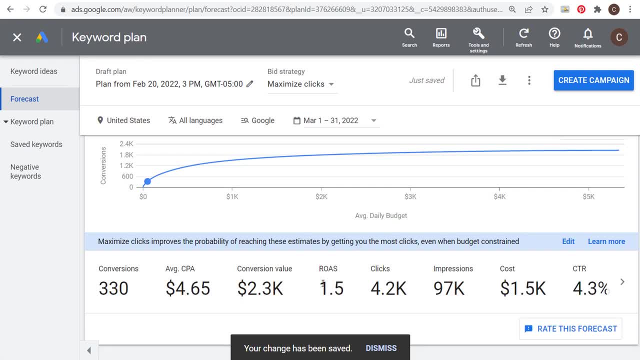 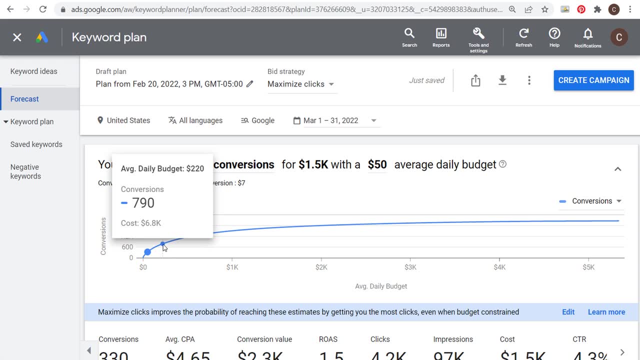 You can adjust all of this data to understand what you're going to get out of your campaign. So in that case my conversion value would be around $2,300.. My cost would be $1,500.. So if you say, okay, I need to drive 1,000 conversions, we click on 1,000.. What you're? going to see here is: my campaign is not going to be profitable if I want to drive 1,000 conversions every single month. But this is all very helpful data to understand where you should set your average daily budget. So a $370 average daily budget not going to be optimal for. 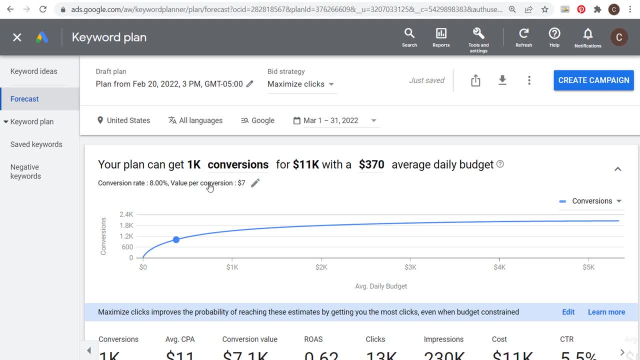 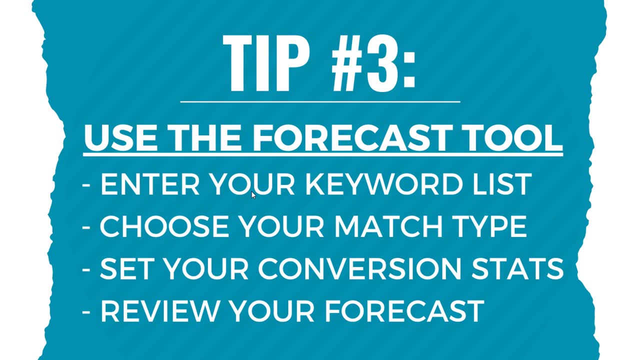 me, but something like $50 might be based on the conversion rate and value per conversion I entered and the keywords I plan on targeting. So tip number three: use the forecast tool to kind of understand what you can get out of a search campaign. Tip number four is going to be a quick. 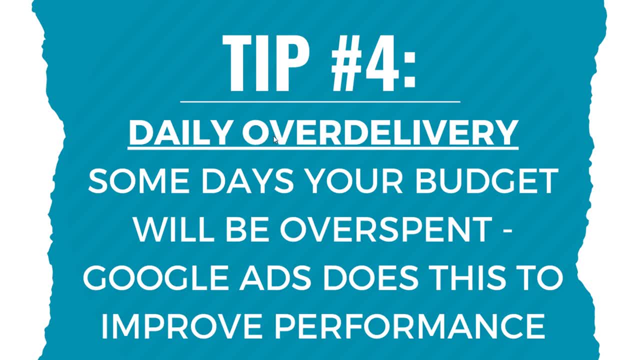 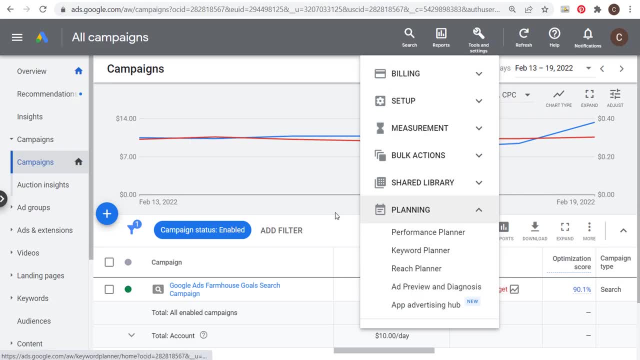 one. I've already went over this. You're going to have some daily over-delivery and under-delivery. Some days your budget will be overspent and Google ads does this to improve performance. So if we come over- you saw, I showed you before- my cost this past Saturday was $13 and 30 cents, And if we just look over, 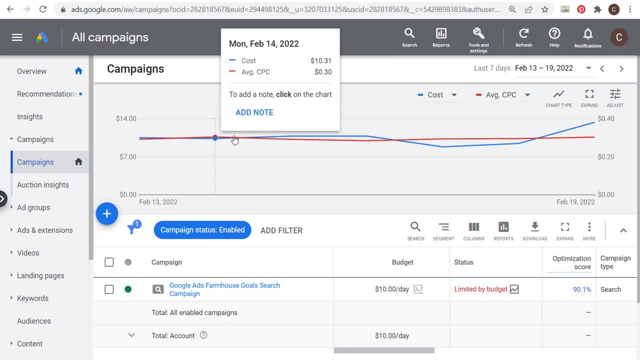 here this past Thursday, $8 and 79 cents. over here we have $10 and 31 cents. So it's going to vary how much of your budget it's Google ads is spending every single day, which is why you don't want to have huge budget swings, because essentially you're hurting your overall performance. 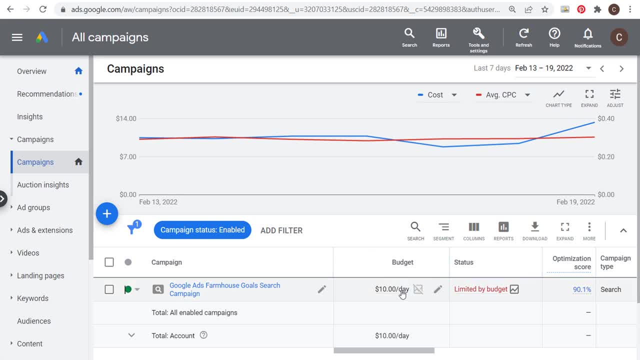 by changing your budget too often. So what I would recommend is, if you do want to change your budget, I would give it at least a week. So up it to $15, give it a week, see how your performance is, Then maybe go up to $20 the following week. You don't. 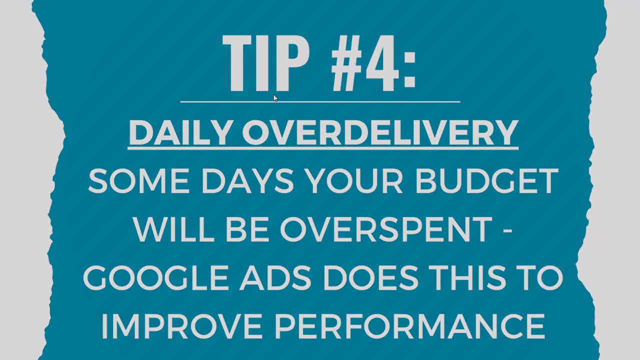 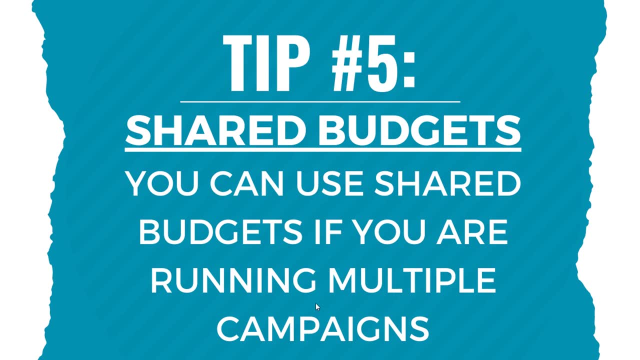 want to have these different swings because you're going to have some daily over-delivery and under-delivery. So tip number five is shared budgets. So you can actually use shared budgets if you're running multiple campaigns. And really to take it a step further, what Google ads? 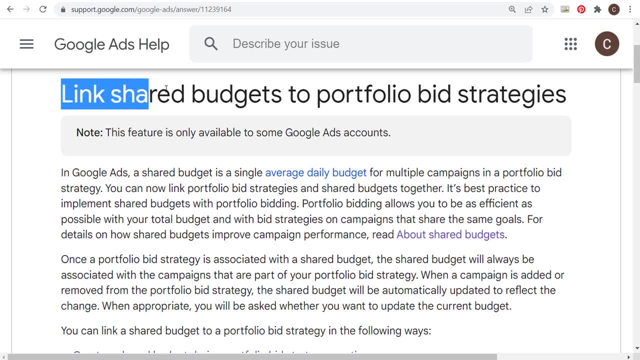 recommends you do if you're using shared budgets is to link your shared budgets to portfolio bid strategies. I'm not going to be going over that in this specific video, but this is the best way to get efficient performance out of your account. I'll put this link in the video description so you 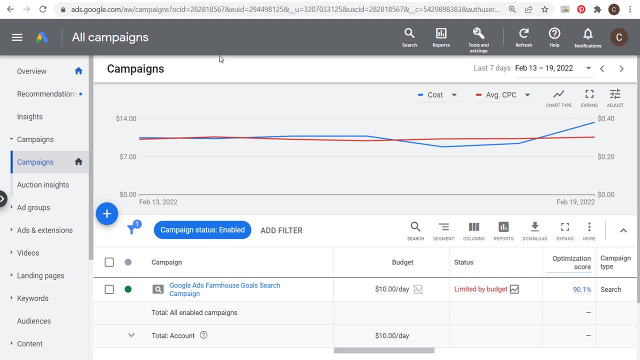 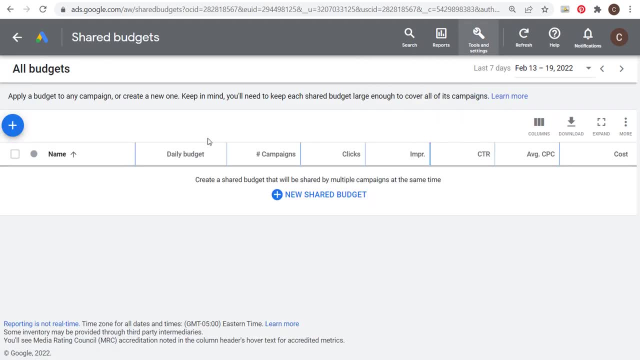 can read more about it. But what you can do is if we come over to Google ads- we click on tools and settings here and we go to shared library, we can click on shared budgets. So in shared budgets we can create a new shared budget. And what we can do here is if we click on this campaign and 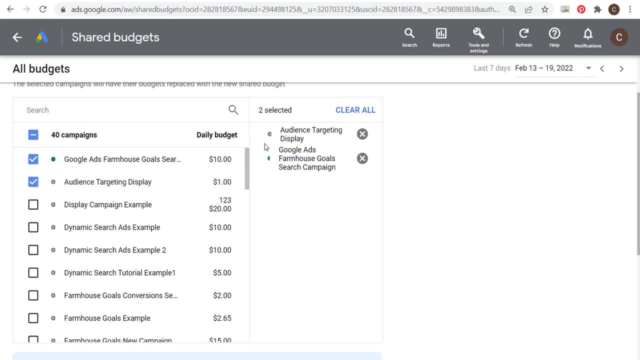 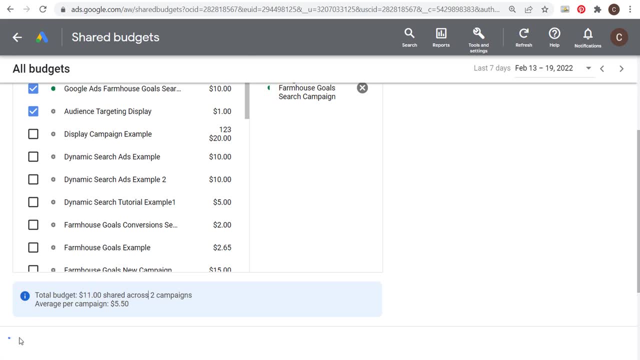 let's just say I want to share this campaign's budget with this campaign over here. I can select both of these and it's going to say my total budget is $11 shared. So we're going to click on save and you can see right here my shared budget example: my daily 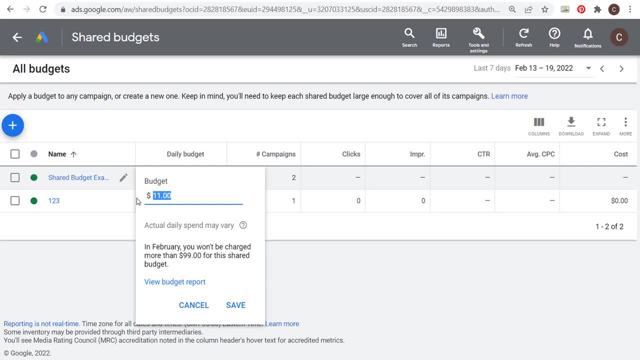 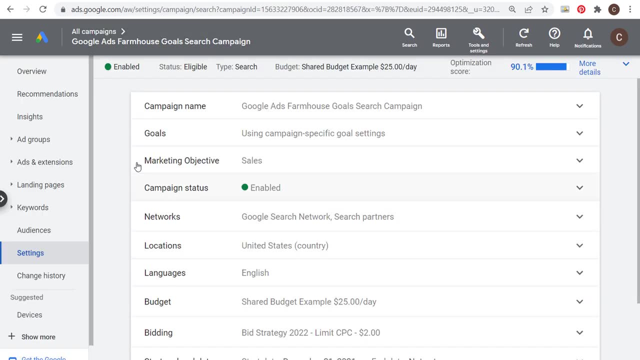 budget $11. So I can adjust this. So let's just say I want to share a budget of $25.. So between those two campaigns my budget is now going to be $25. So I would obviously have to activate the. 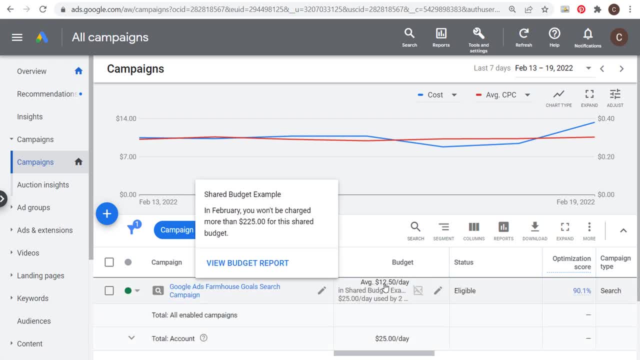 other campaign. But if we come back over to my campaigns, you can see my average is $12 and 50 cents per day for this campaign. But what's going to happen is if one campaign is under spending, then Google ads will spend more on this campaign. 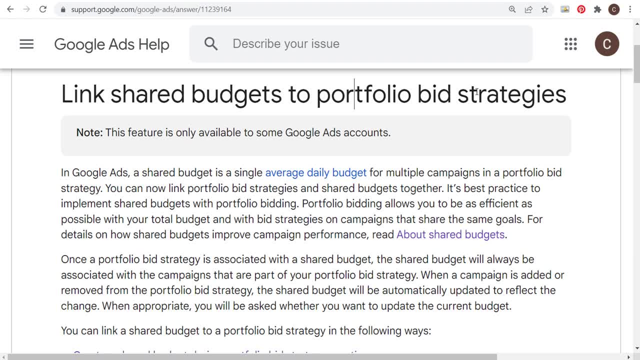 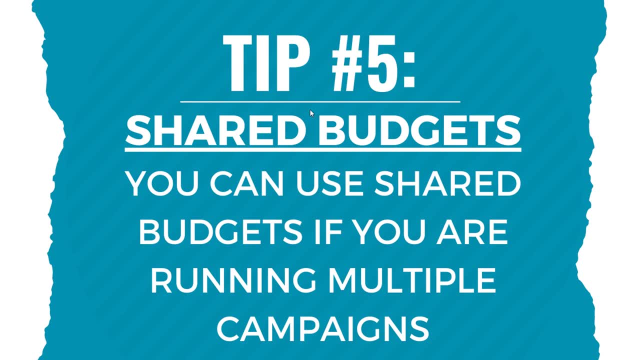 So Google ads will recommend budgets that can help you improve your performance. So, if you're using a shared budget, you can use shared budgets to make sure that you're spending a minimum amount of $25 per day- $50 per day- even if it has to be split between different campaigns. So that's. 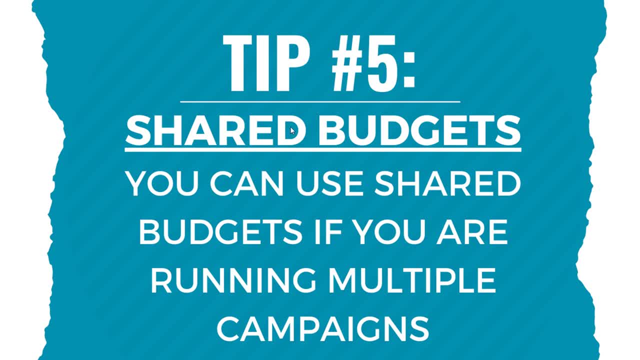 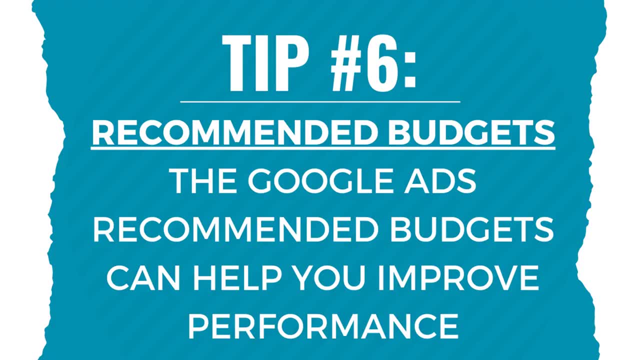 another option you have when you are setting your budgets and trying to figure out how much you're spending on different campaigns. Okay, So tip number six recommended budget. So Google ads will recommend budgets that can help you improve your performance. So let's come back over to our 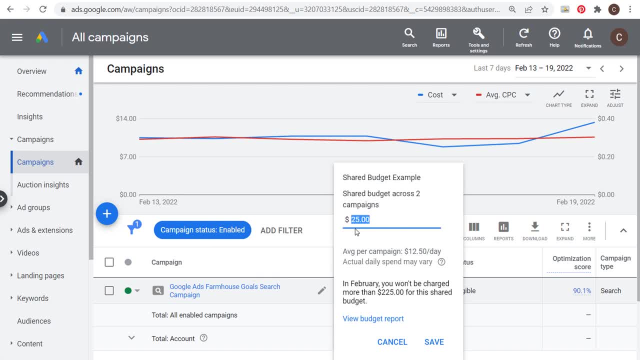 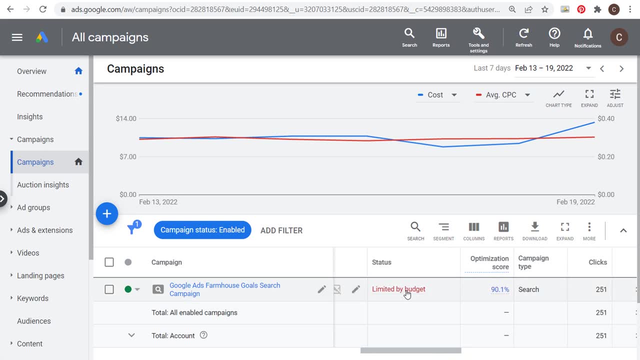 campaign here and let's just come back to our standard $10 budget. Okay, So I went into settings and just set this back to $10 per day And you can see my status is limited by budget. So what you can do is click on limited by budget. So if you come over here and this actually just got rid of my 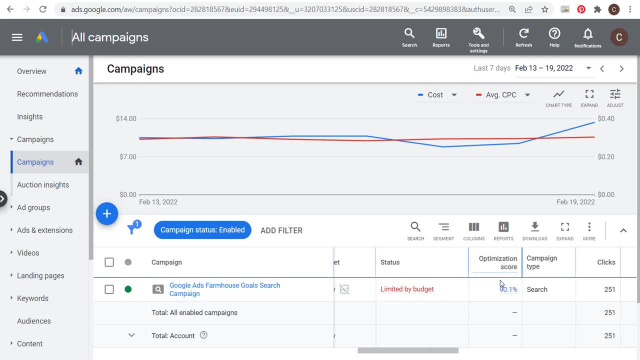 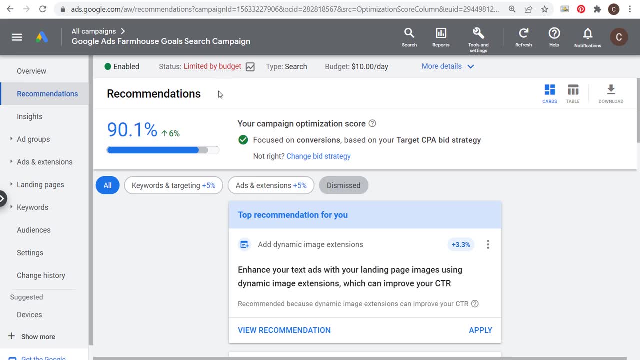 option to look at the best budget for my campaign. But if you do go to optimization score, you click on your optimization score here you're going to see limited by budget at the top- If you do have a page there- and you're going to see this little graph icon: the budget Explorer. So when you click, 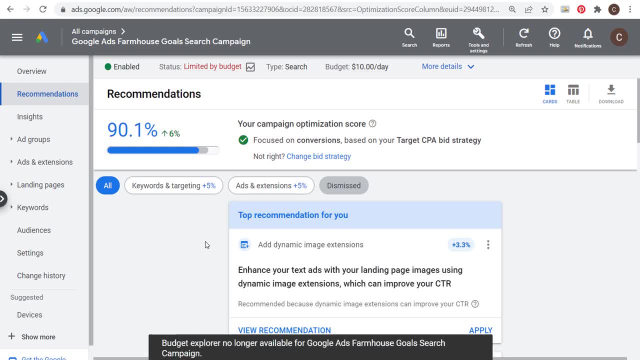 on budget Explorer. you're going to see I get an error message at the bottom here, but as you collect more data for your campaign- and obviously this is why you don't want to change your budgets all the time- When you do click on this it's going to bring up a graph and set a recommended 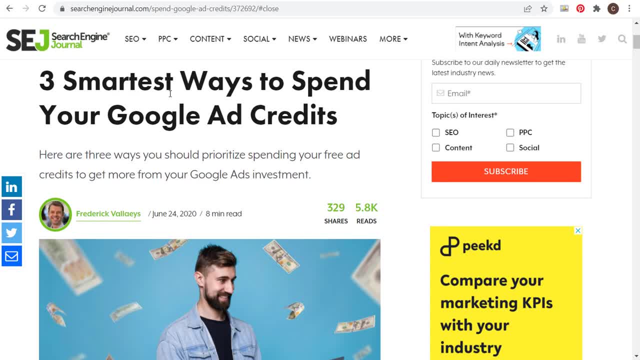 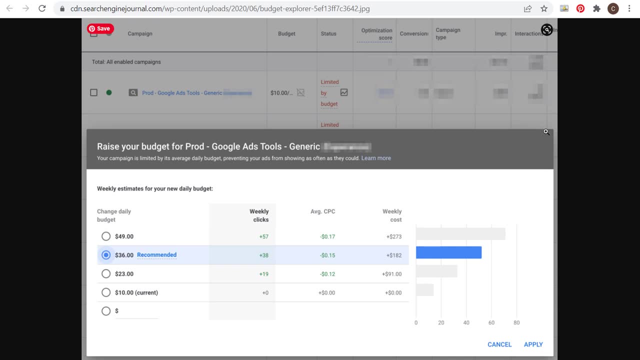 budget for you. Now, just to give an example of budget Explorer, I found an example in this article: three smartest ways to spend your Google ad credits on search engine journalcom. So if we open up the picture, when you do click on budget Explorer, it's going to open up a prompt that looks like this one here: 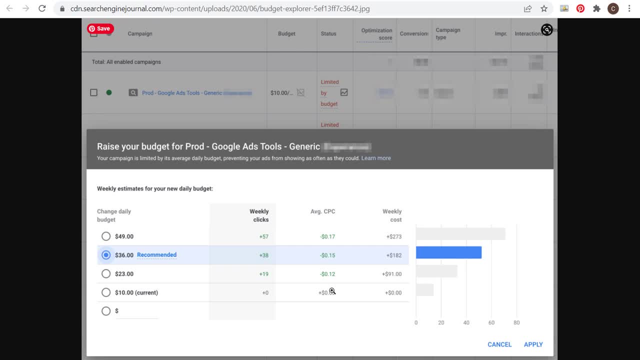 at the bottom, where you can see their current budget is $10. Actually the same one my campaign is, So $10, they show a $23 daily budget. We'll add 19 clicks, lower the average CPC by 12 cents and the weekly costs will be 91 additional dollars. And then, if they go up to a daily budget, 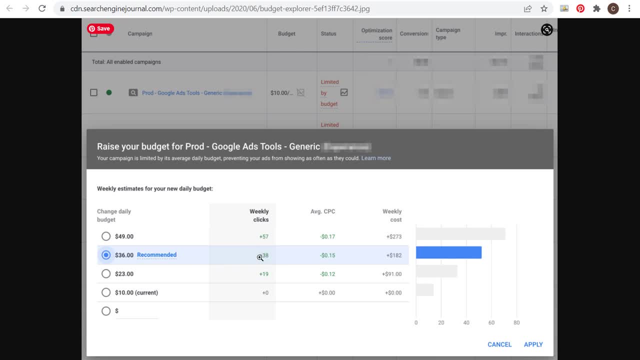 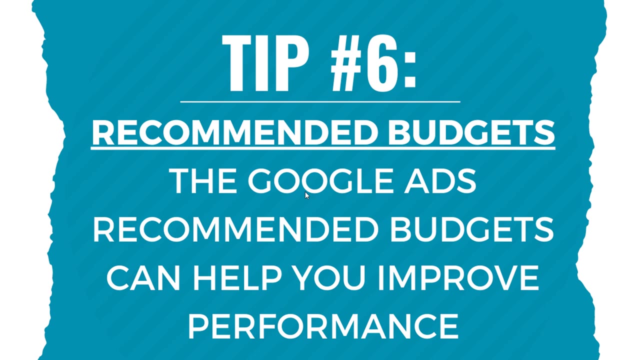 of $36, which Google ads recommends. it'll add 38 clicks, drop the average CPC by 15 cents and add a weekly cost of $182.. So just wanted to give a quick example of what the budget Explorer looks like. So, using recommended budgets, the more data that Google ads gathers, they're going to say: 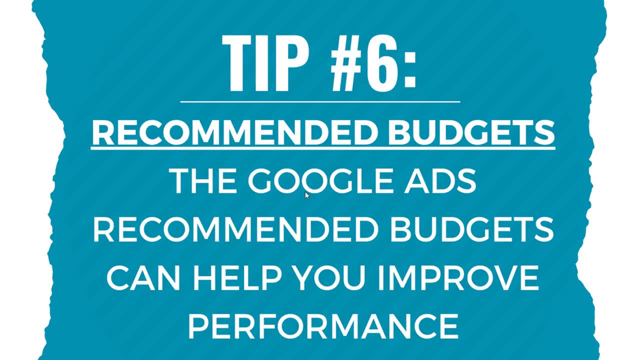 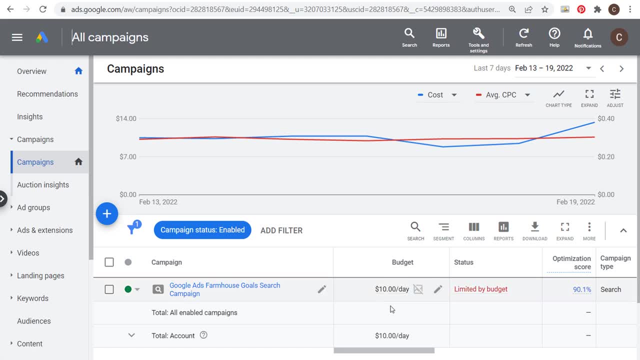 okay, we can drive the same amount of conversions at the same cost up to this daily budget. So, for example, if I'm only spending $10 per day, but Google ad says, if you spend $25 per day, you're going to get the same exact performance, That's what you're going to see when you do click. 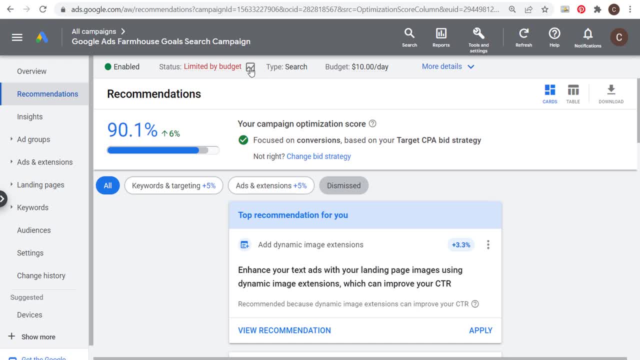 on limited by budget here, or you click on the optimization score And click up here on the graph. that will show you what the optimal daily budget is for your campaign, As long as you're kind of looking for the same exact results, And then you can also see how your 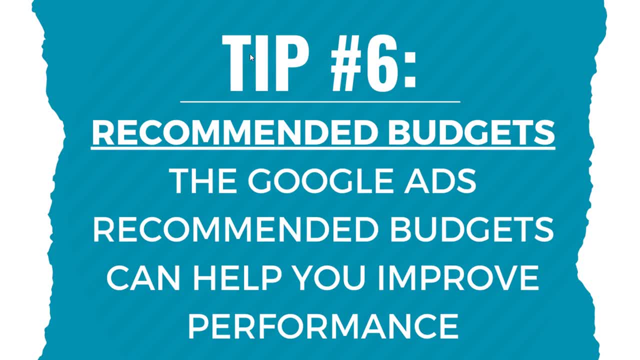 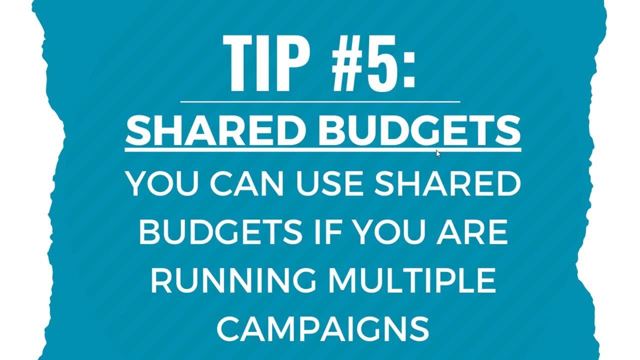 campaign will perform with higher or lower budgets, So another option is to use recommended budgets. If I didn't change my shared budget or my shared budgets in the previous step, I would be able to show you how mine looked, but it recommended a daily budget of $14 for me. So basically that. 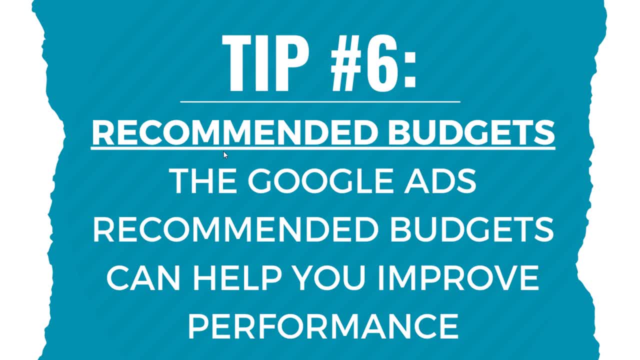 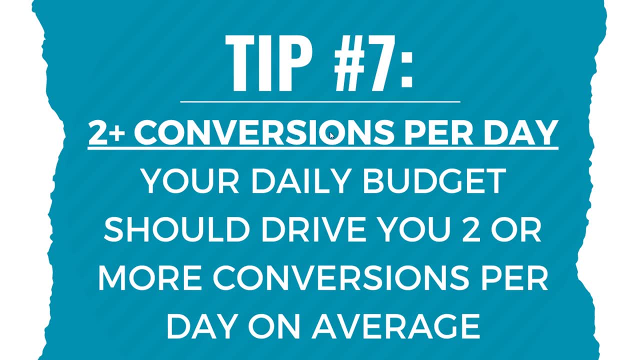 means they can drive the same performance At $14 per day as they do at $10 per day. last but not least- and this is really more of a personal preference here, but what you're trying to do is, on average over the course of a month, you should. 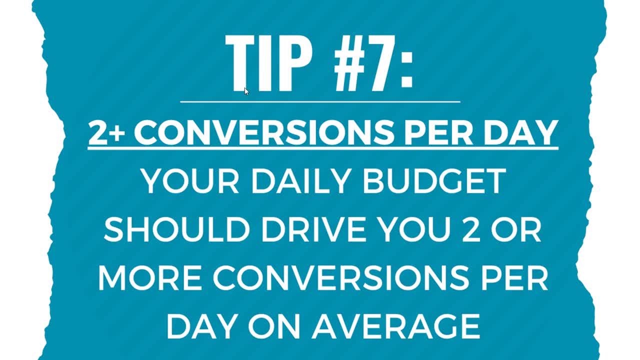 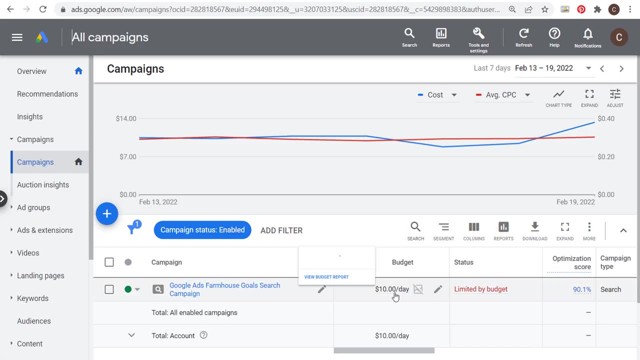 be driving two plus conversions per day, So basically over a 30 day period. if you're driving at least 60 conversions, that allows Google ads to really optimize your campaign much better than if, for example, you're driving 20 conversions over a 30 day period. So what you want to do is you see. 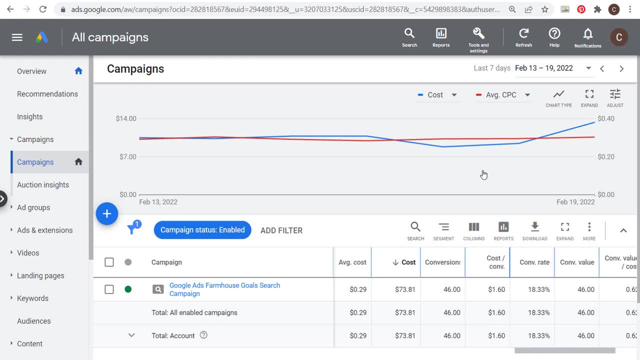 my budget is $10 per day. If we come over here and you can see my cost per conversion over the previous seven days is $1.60.. If I set my daily budget at $3 per day, I'm only driving maybe one, maybe two conversions every. 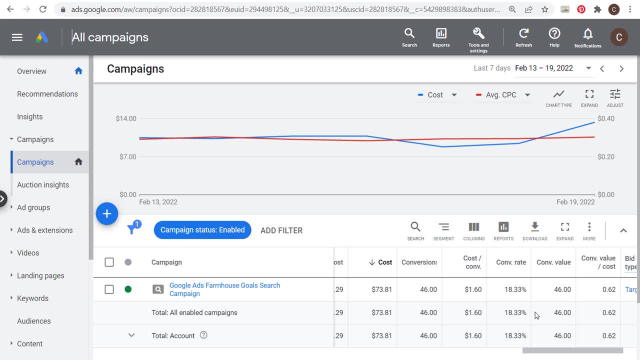 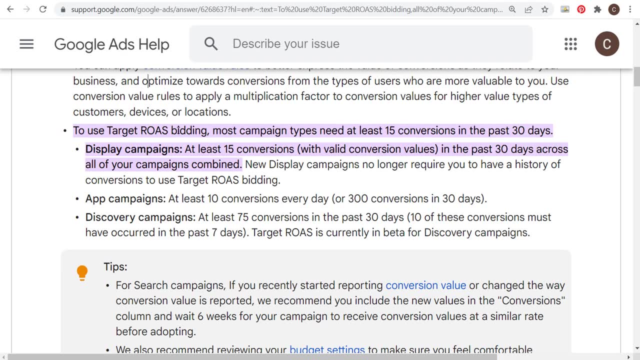 single day, So it's much more difficult for Google ads to optimize my campaign. Then, for example, if I'm driving 46 conversions over a seven day period, if you're using target return on ad spend bidding, most campaign types need at least 15 conversions over the past 30 days.